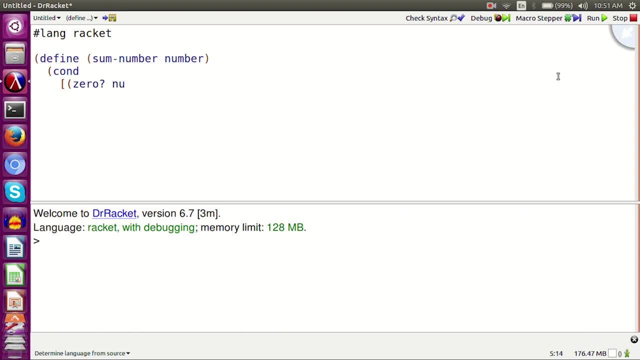 example, 3 should return 3 plus 2 plus 1 plus 0, which is 6. 0 should return 0.. Define some number, number. Cont 0 number 0.. Else plus number some number sub 1 number. Write a function. 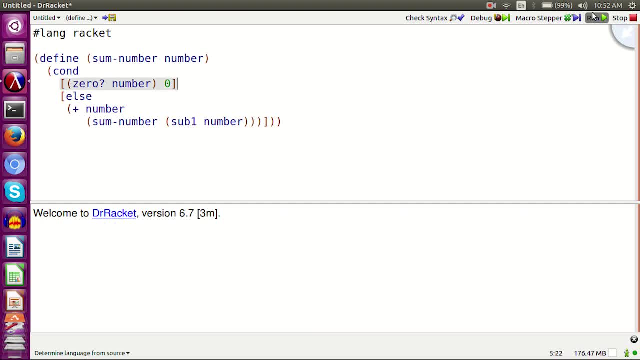 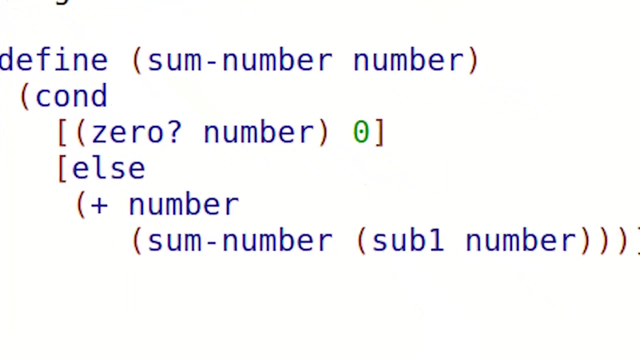 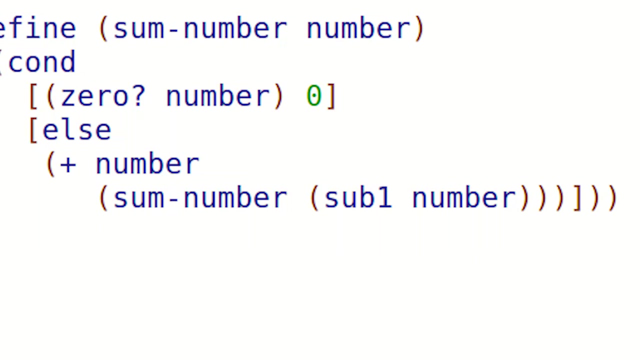 number, Some number 3.. Some number 6. Some number 10.. First part of cont is the base case of this recursive function. Else part is the recursive case. Some number sub 1 number is the recursive function call Recursion in computer science is a method where the 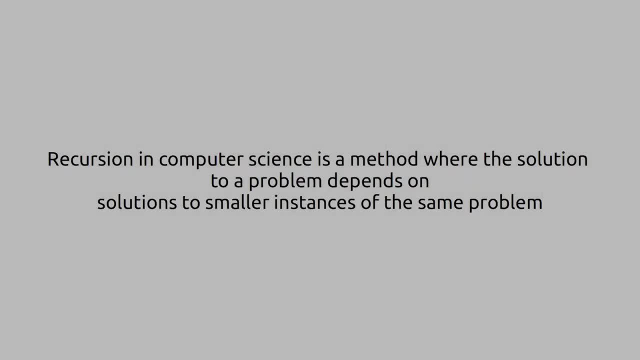 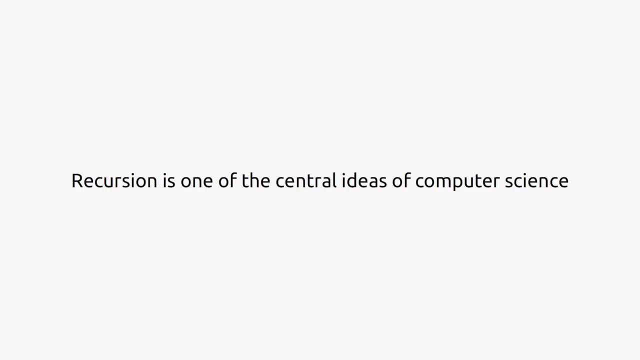 solution to a problem depends on solutions to smaller instances of the same problem. Recursion is one of the central ideas of computer science: Factorial function. Factorial is the product of all the positive integers from 1 to n. For example, 0 to n is the result of: 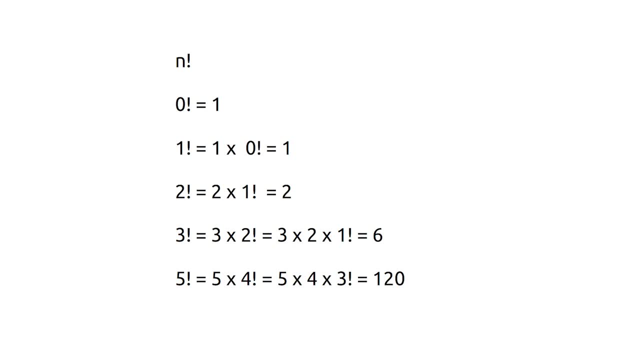 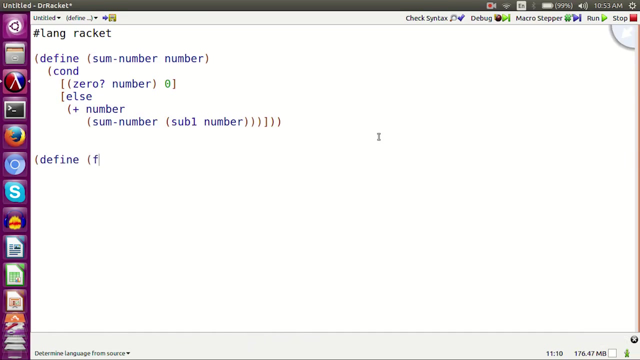 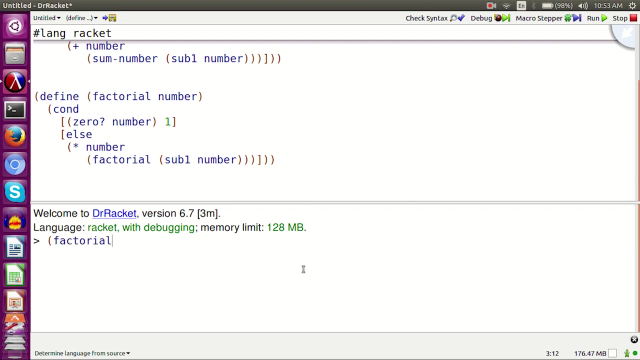 all the positive integers of the same factor. It must be also posittional. 0 is the result of all solutions. Well, that was a simple refinal, This asterisk number factorial sub 1, number factorial 3, factorial 0, factorial 5.. 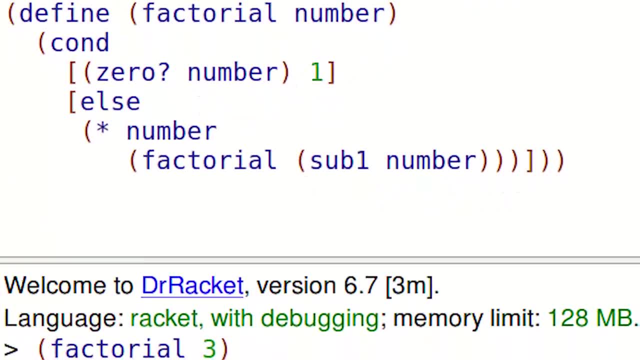 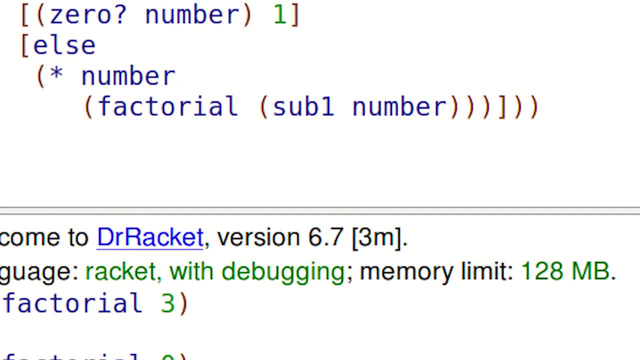 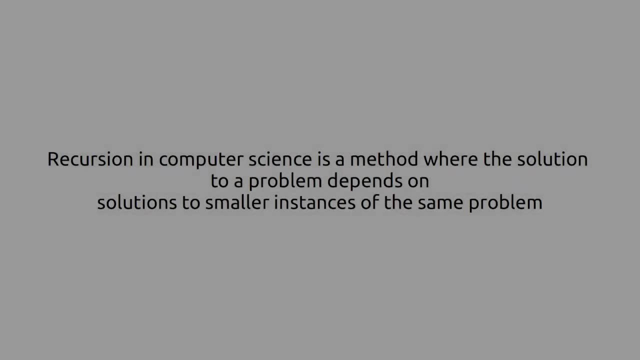 First part in the cont is the base case. else part is the recursive case. Factorial sub 1 number is the recursive function call Recursion in computer science is a method where the solution to a problem depends on solutions to smaller instances of the same problem.